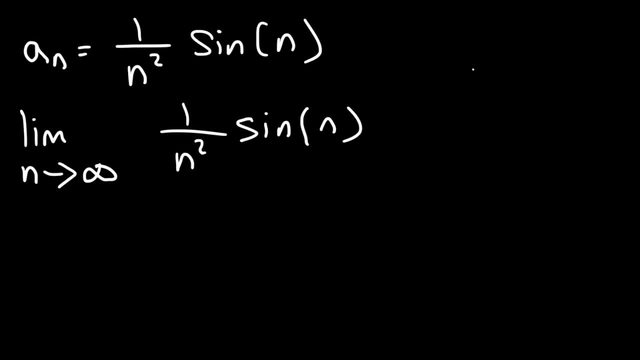 Now we need to be familiar with the behavior of sine. So let's say, if we were to graph sine x, This is basically a sinusoidal function that varies between 1 and negative 1. So we could say that sine n will always be between. 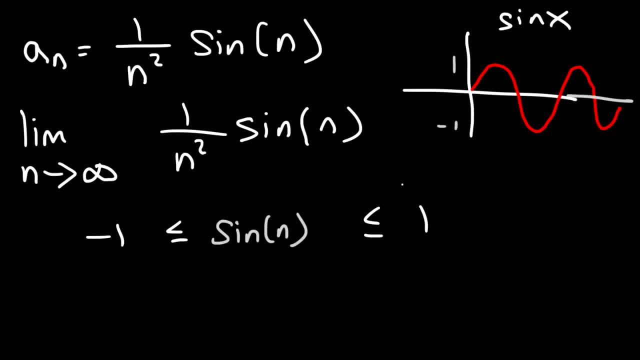 negative 1 and 1.. Now, taking this expression, let's divide all three sides of the inequality by n squared, So we're going to have negative 1 over n squared, sine n over n squared, which is the original expression. 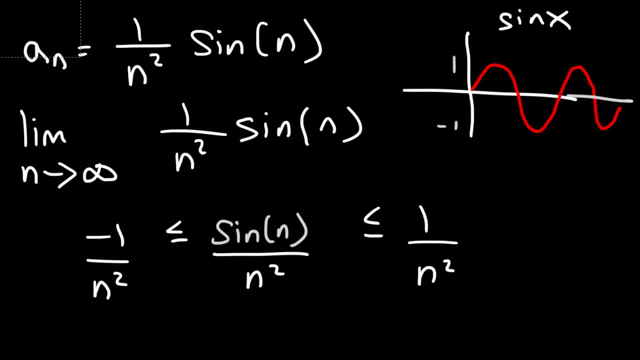 and positive 1 over n squared. So now, in this form, we can apply the squeeze theorem. So what is the limit, as n approaches infinity, for negative 1 over n squared? Well, we know that's going to be equal to 0.. 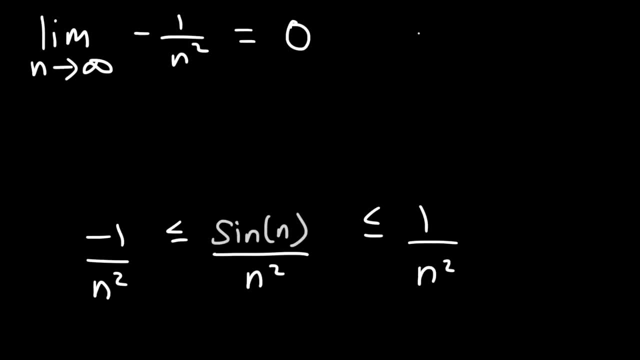 Negative 1 divided by a very large number will give you a small number. Likewise, the limit as n approaches infinity. for positive 1 over n squared is also 0. So because these two limits equal the same value, then for the function in the middle we should also get the same value as well. 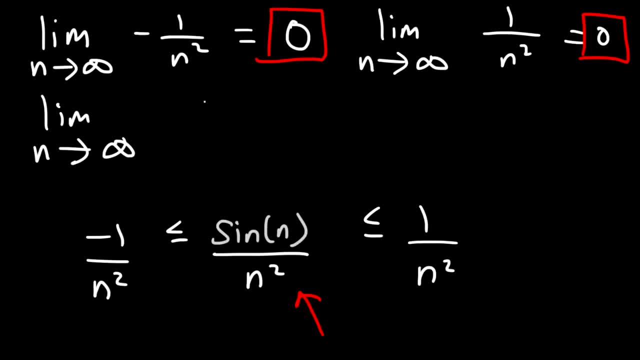 I mean the sequence in the middle. So the limit as n approaches infinity for the sequence sine n over n squared must also be 0, based on the squeeze theorem. And so that's how you can use the squeeze theorem to determine if a sequence will be. 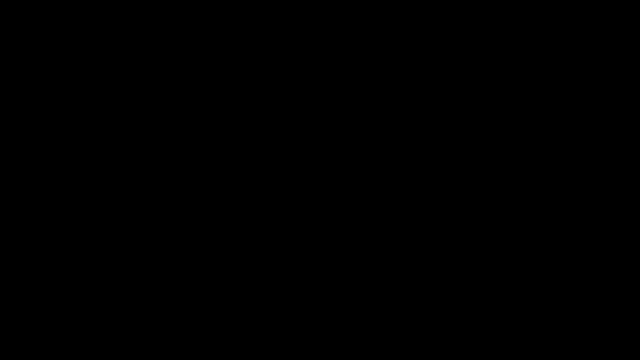 if it's going to converge or diverge. Another way in which we can determine if the sequence is going to converge or if it's going to diverge is to graph the sequence as a continuous function. So let's say, if we have the function f of x, 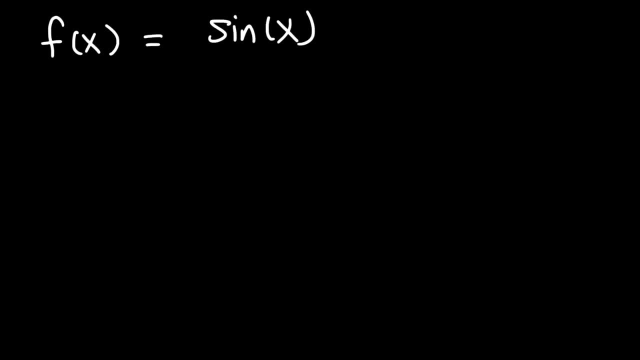 and we're going to say that's equal to sine x over x squared. Go ahead and graph this function in your graphing calculator, Or, if you don't have one, just use an online graphing calculator. So if you graph this function, it's going to look something like this: